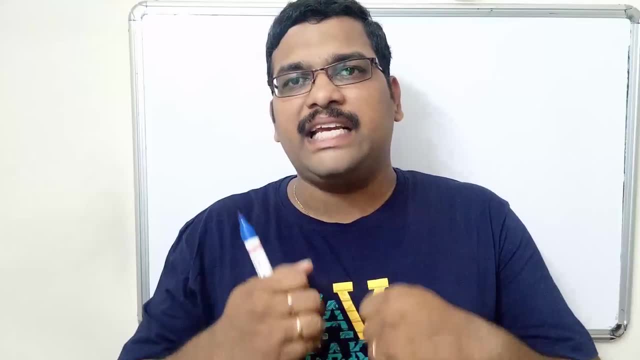 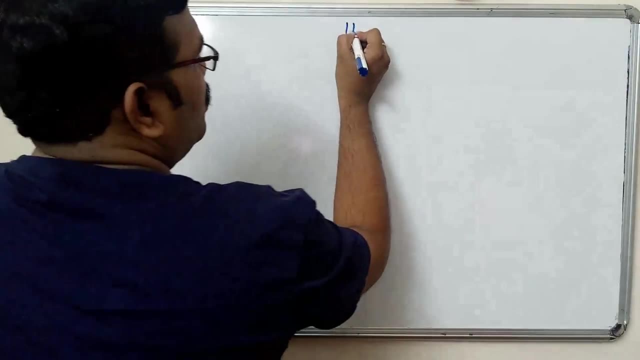 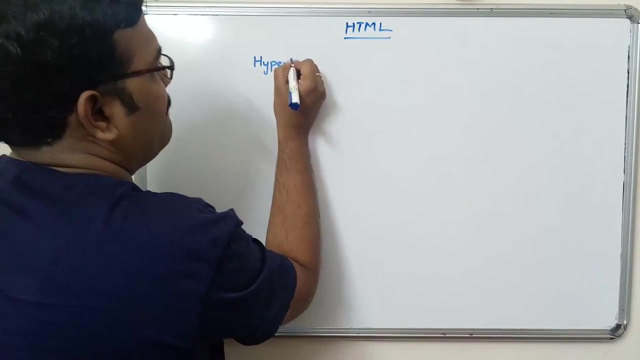 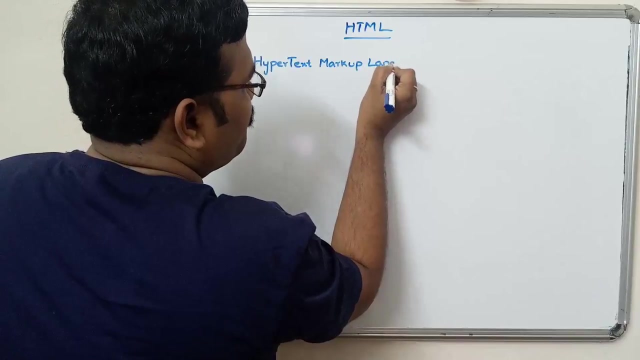 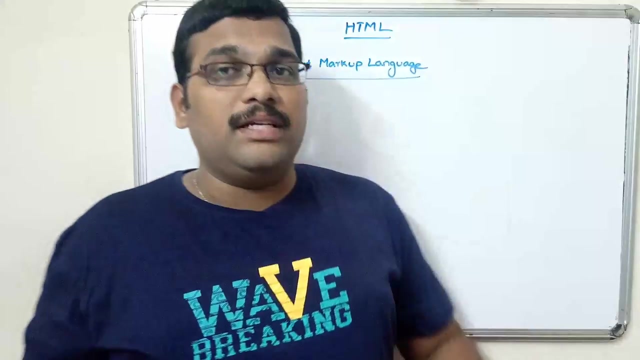 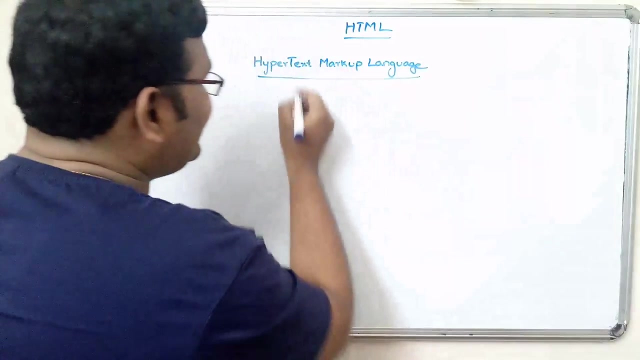 to create these websites, the basic need or the basic requirement is HTML, So HTML is HTML. HTML stands for hypertext markup language, So here I mentioned it as a language. don't think it as a programming language, right? It's a markup language, So this is used to. 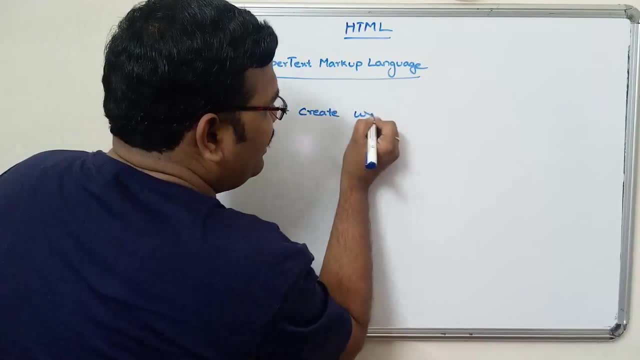 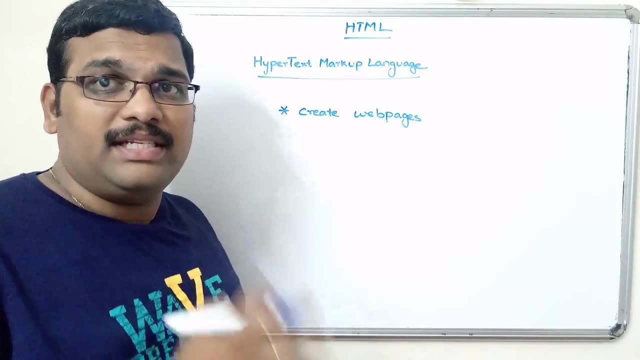 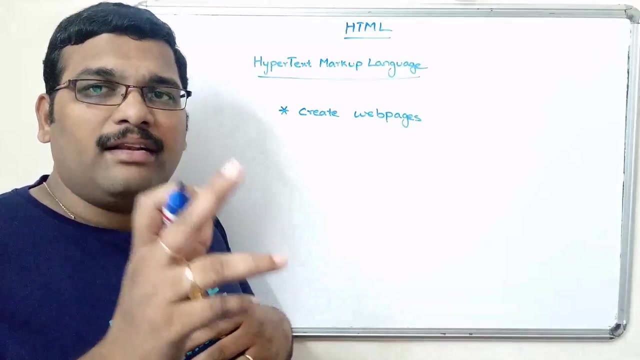 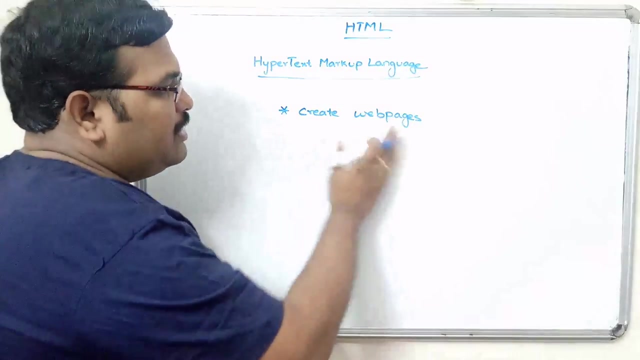 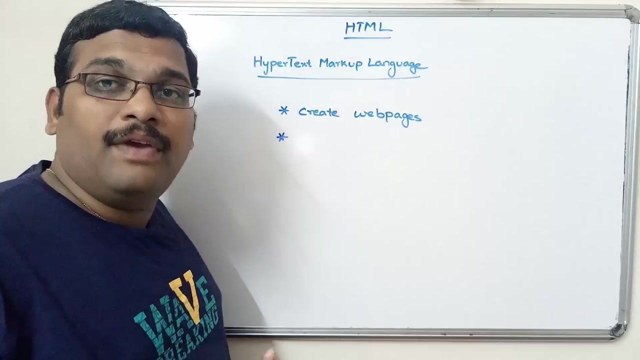 create a website. Create web pages Definitely. after this session- I mean after this course, this HTML and JavaScripting- I promise that you can create a simple website on your own. So this is for creating a web page Then, where we will use this. 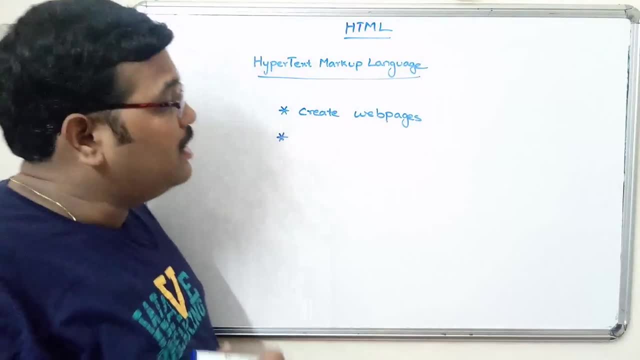 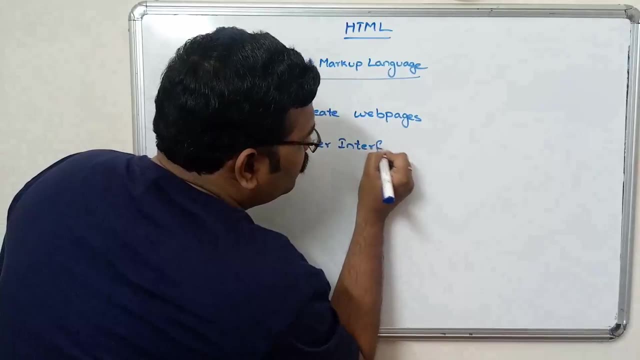 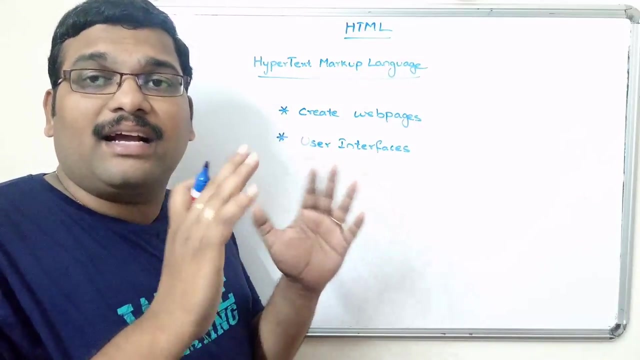 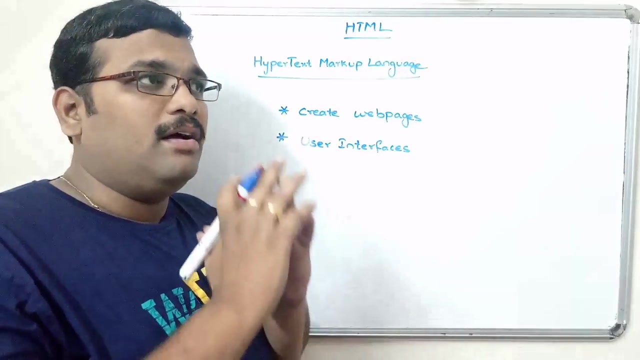 Hypertext markup languages And this is used to create user interfaces. User interface means if you open a website so we can see the color background, the text font, the text size, the paragraphs, the alignments and everything. Simply, we can say it as a look, and feel, look. 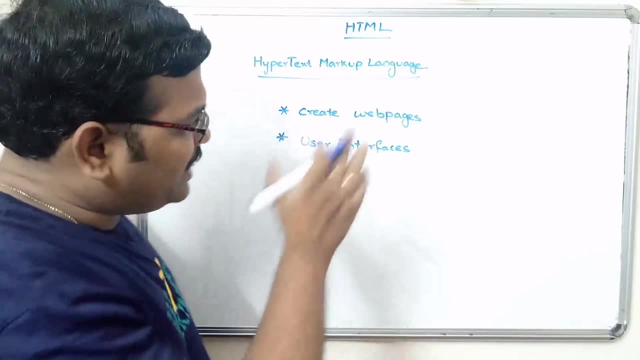 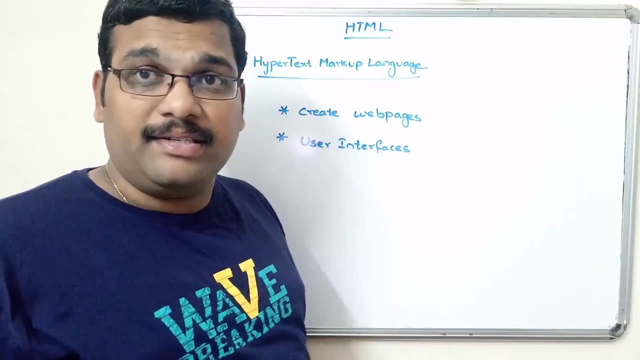 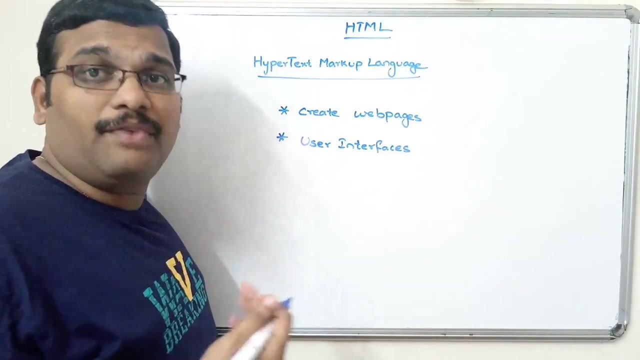 and feel first impression. right, so that can be achieved by using hypertext markup language. right that we call it as a user interface. next, so what is the requirement for this? so what is the software we need to implement this html? so there is no explicit software required to implement this. 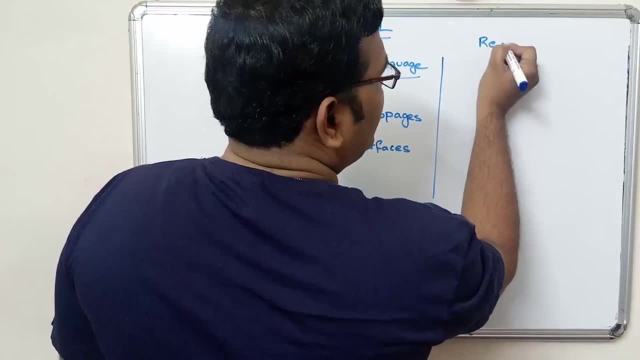 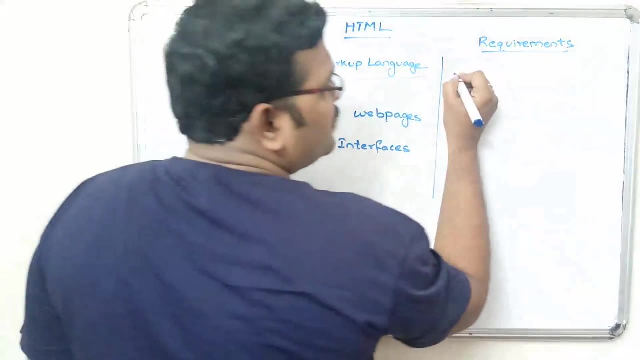 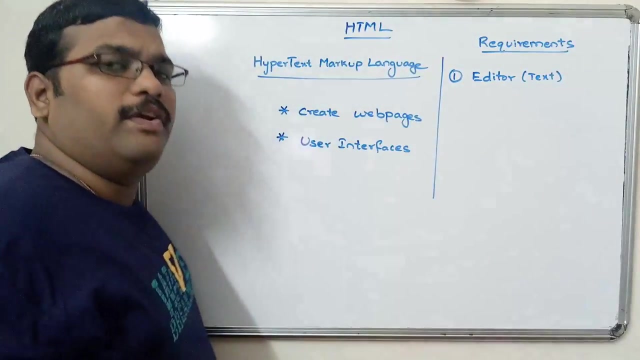 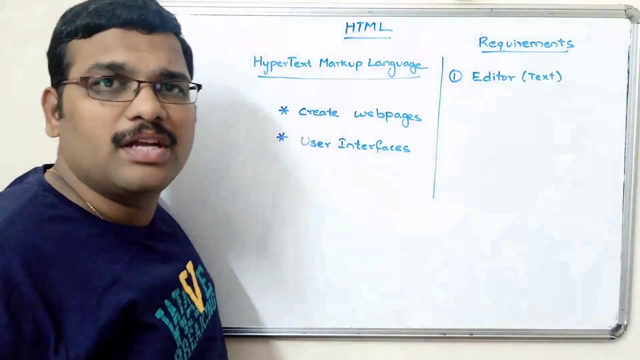 html we need. so these are the requirements: see requirements to implement this html. the first one is editor. it's a text editor, so we can use a notepad also. right, we can use a notepad because it is an a text editor- any text editor we can use to create HTML web page. second, 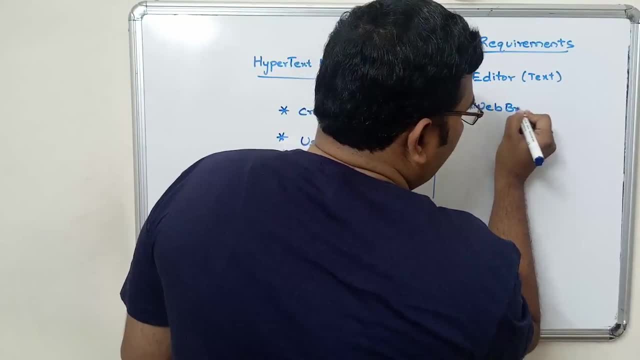 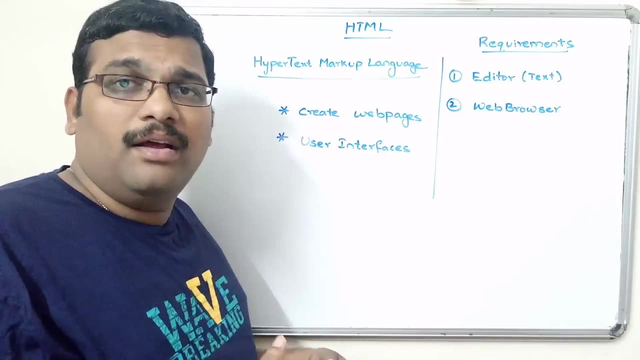 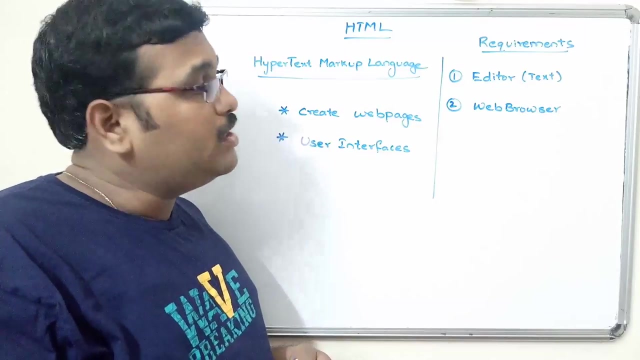 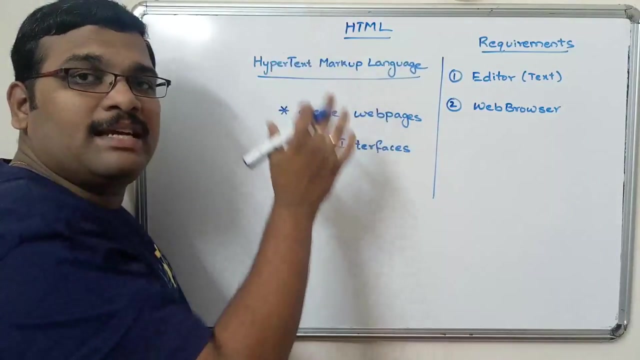 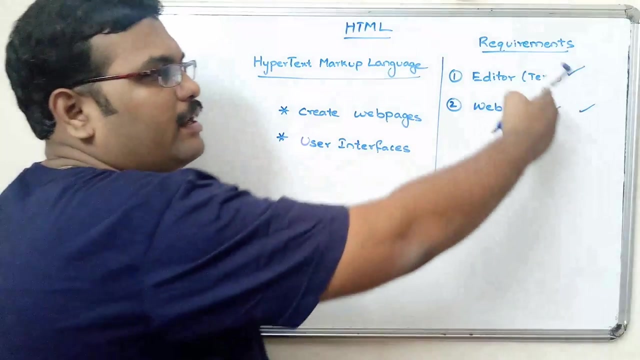 is webcage browser. i think all of you are familiar with this web browser: internet explorer, google, chrome, netscape, navigator, modulo, firefox, opera. so all these are the web browsers available. so we can use any one of the web browser. so the requirements to implement these html or creating these web pages is only the editor and the web browser. so editor is. 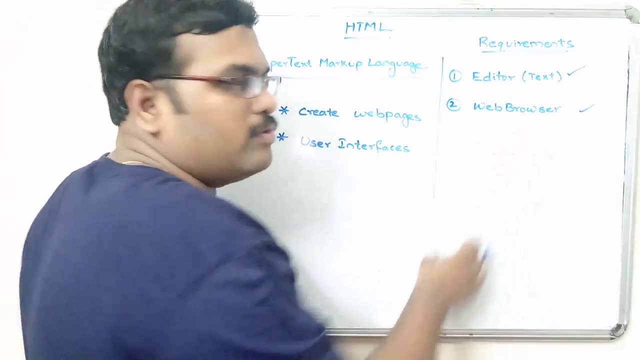 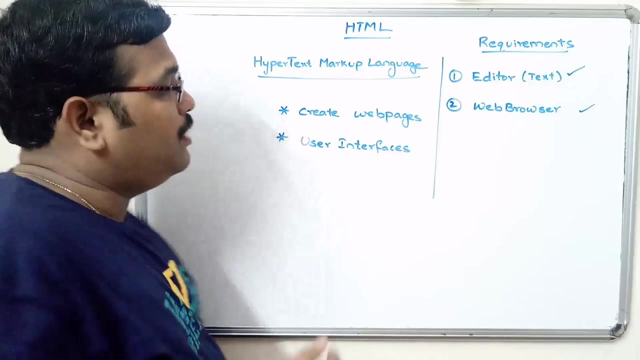 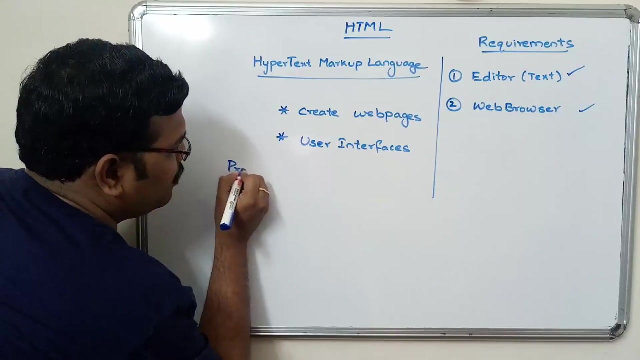 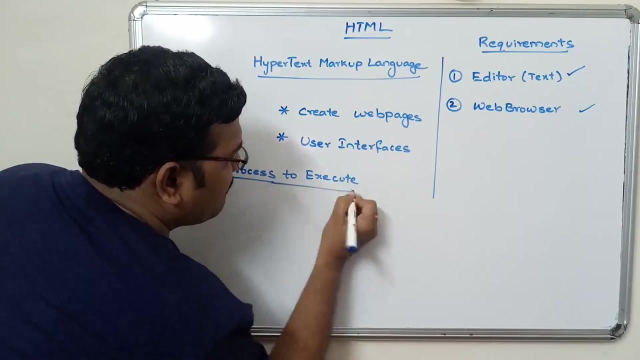 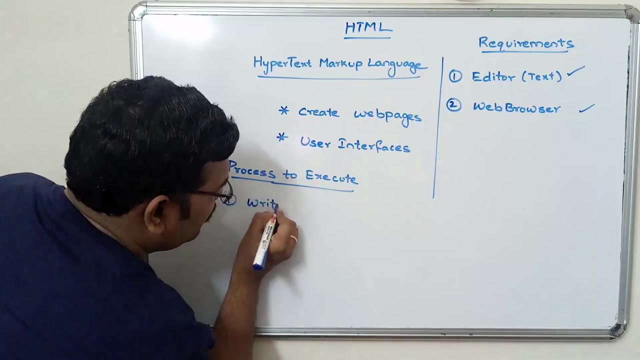 written meaning. this is not really a service. it's nice but familiar with it. it's just a plain user to write the HTML tags and web browser is used to implement the HTML code. next process to execute first one, we have to write the code in text editor: write HTML. 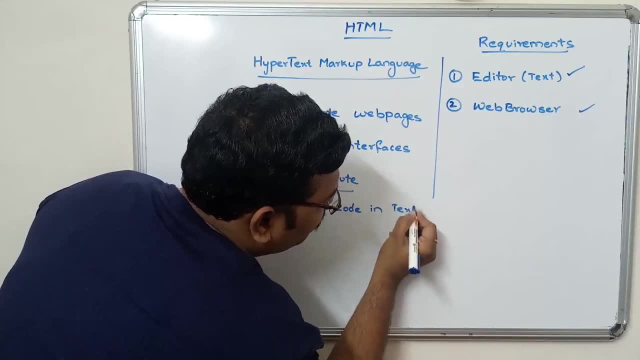 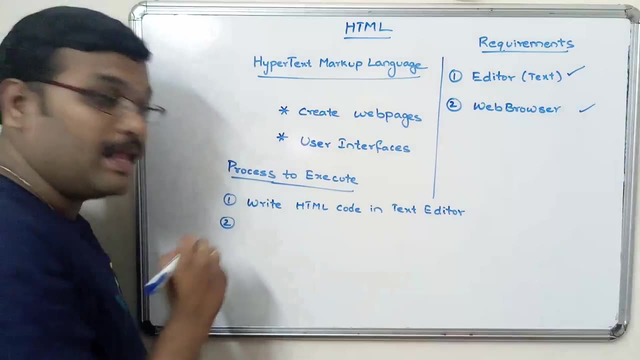 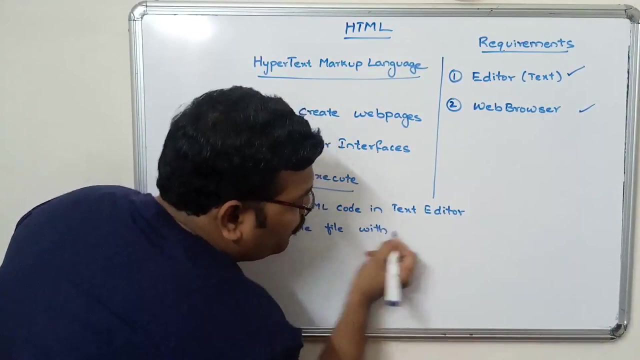 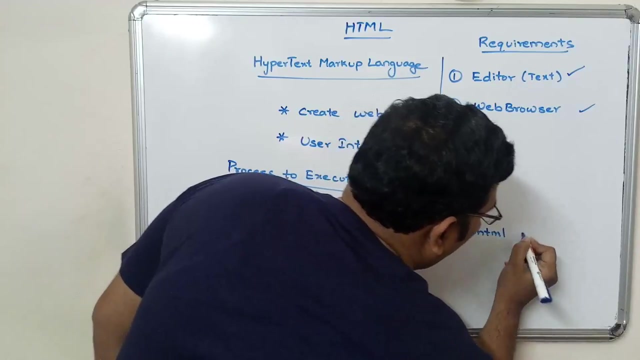 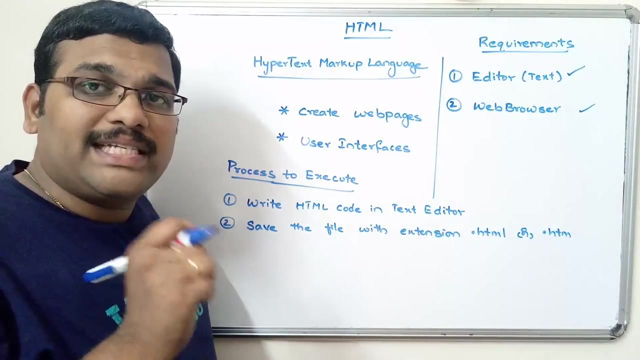 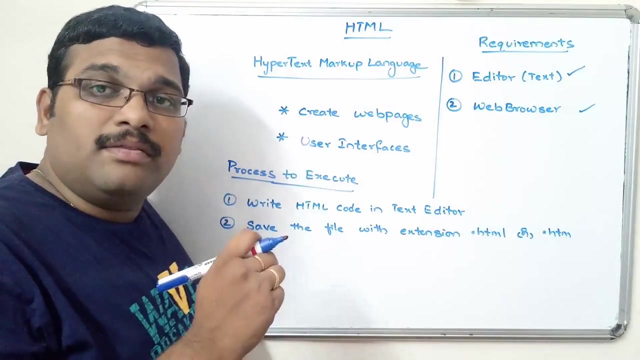 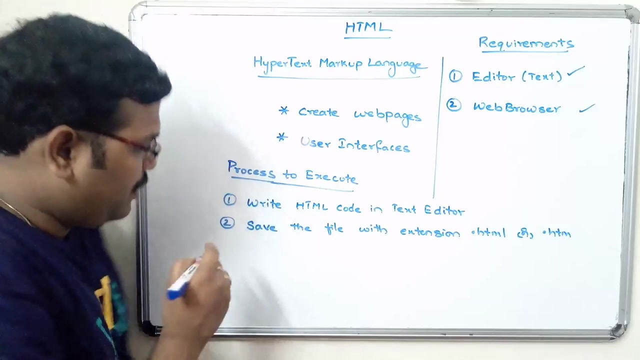 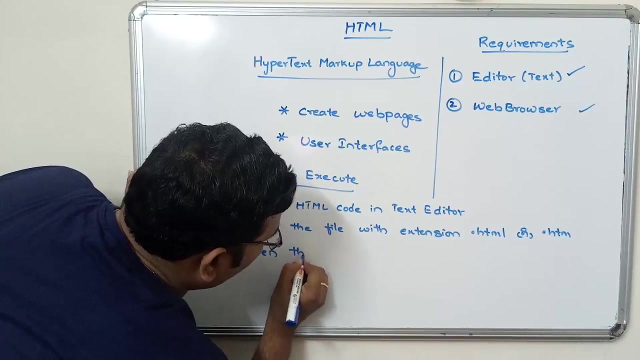 code in text editor of your choice, anything same. second: save the file with extension HTML or HTML. so if you save the particular file using HTML or HTML, that implies that is a web page. that's not a file, it's a web page. third one: open the file. 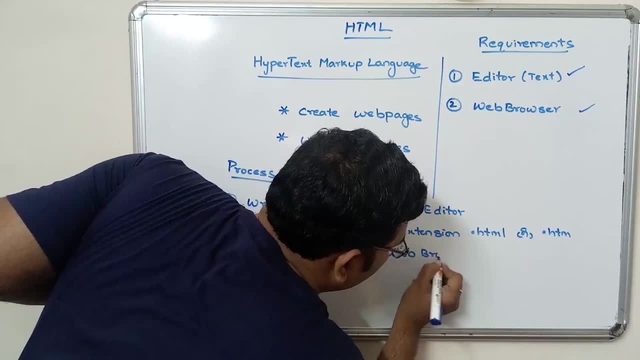 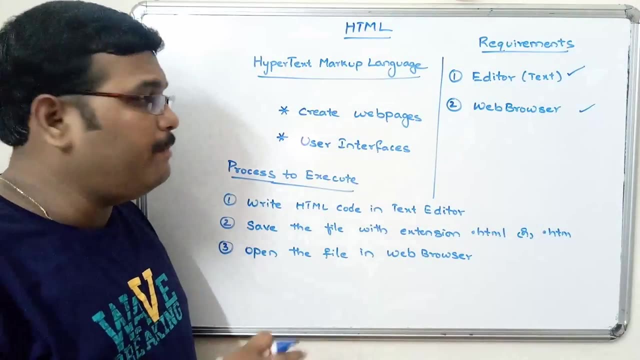 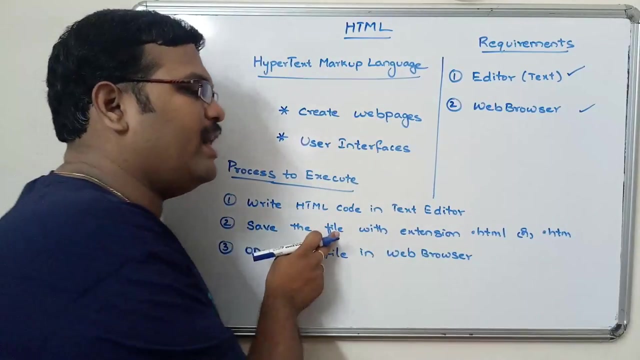 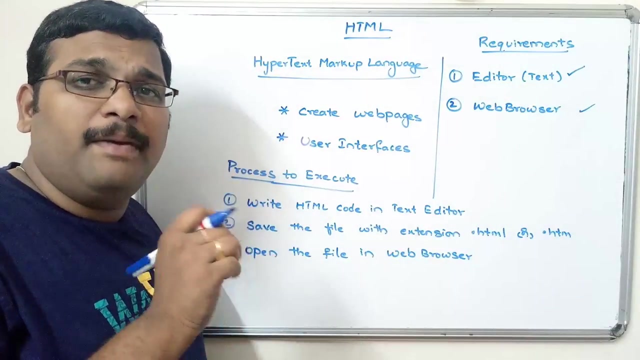 in web browser. simple thing, only three process, three steps in order to implement any HTML web page. so first, we have to write the HTML code in text editor. second, you have to save the file with extension HTML or HTML right. so for every file there will be an extension. so whatever the file we are saving in the 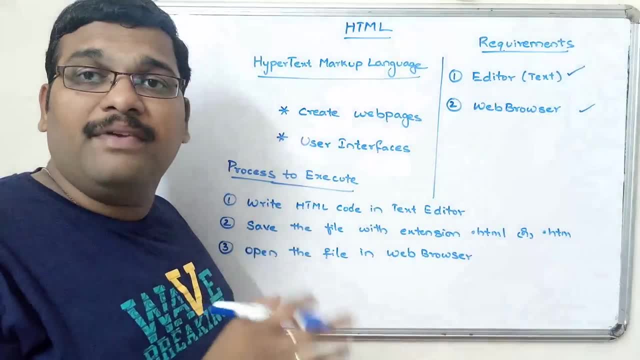 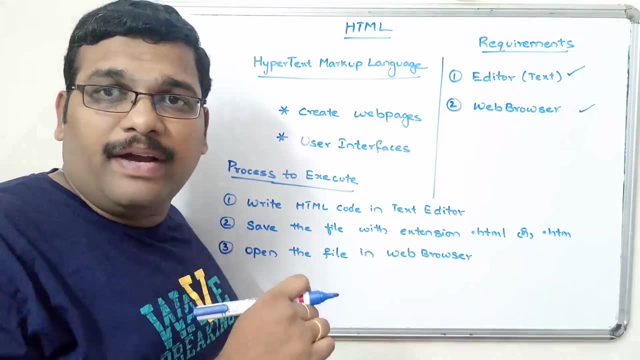 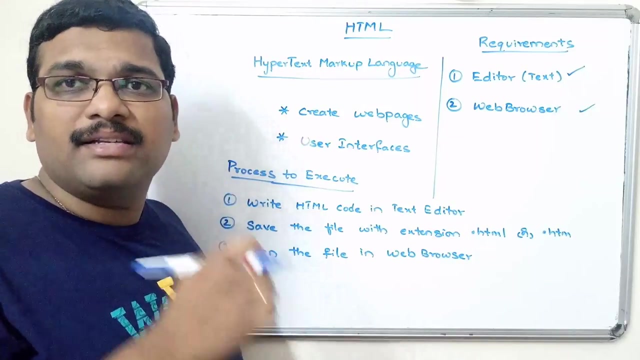 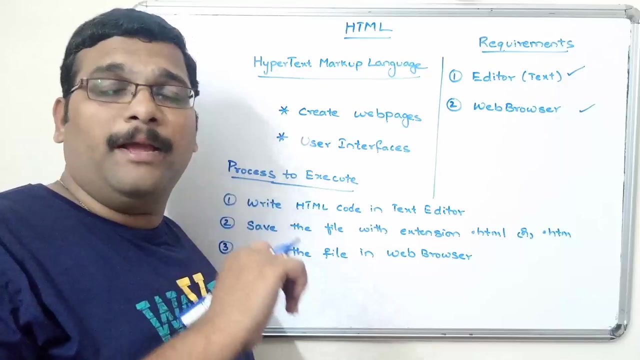 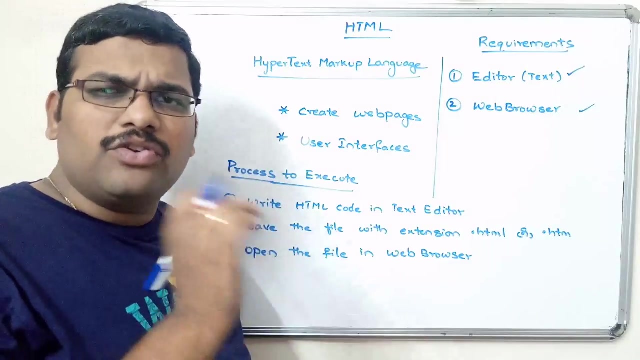 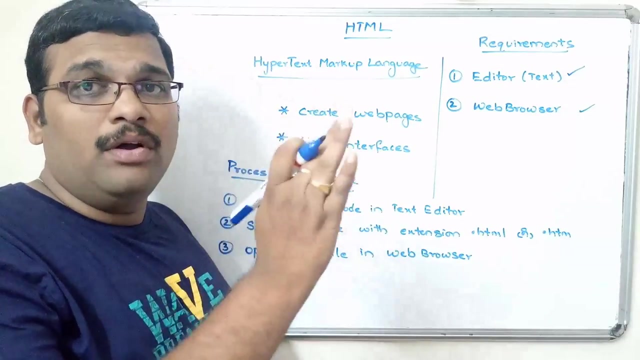 computer, it will be having one extension. so for the C programming files, the extension is dot C. for Python programming files, the extension is py. the document, the document files, the extension is doc. text files, the extension is txt. multimedia files, that means songs, the extension may be mp3 or mp4, and the video files, the extension will be mp4 or vob. so like that, every file in our system will be having an extension. so by seeing that extension we can know that what type of data is available in that particular file. 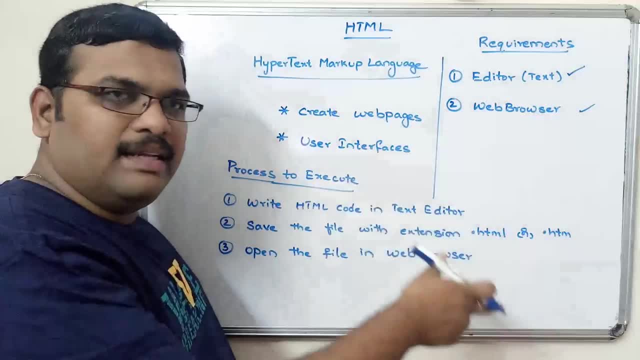 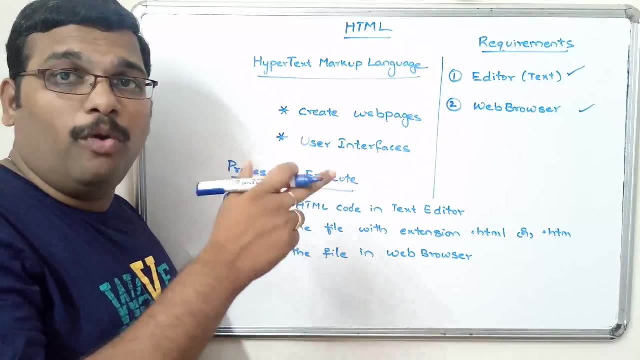 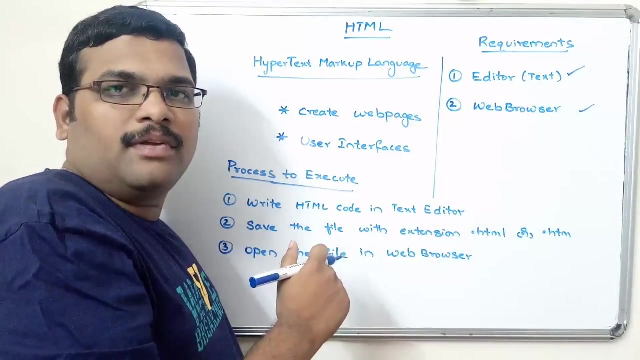 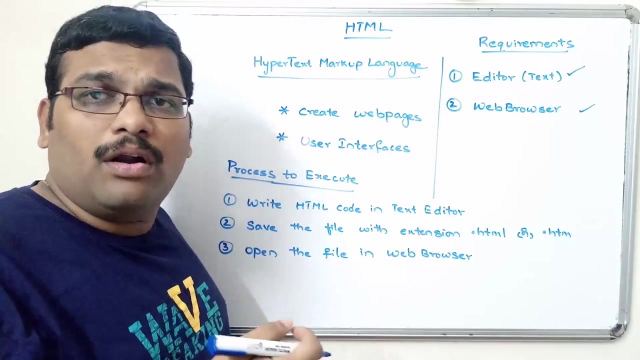 similarly here. if the any file is having the extension html, or html, that implies is a web page, so it will be opened in web browser. so first of all we have to install this web browser right? so I think in every system you can find this web browser: either Internet Explorer or the Google Chrome, anything, any web browser, right? 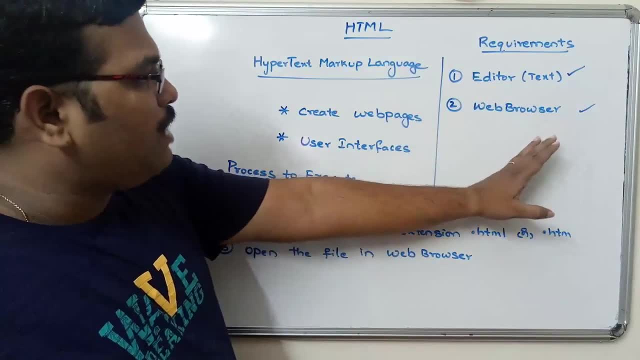 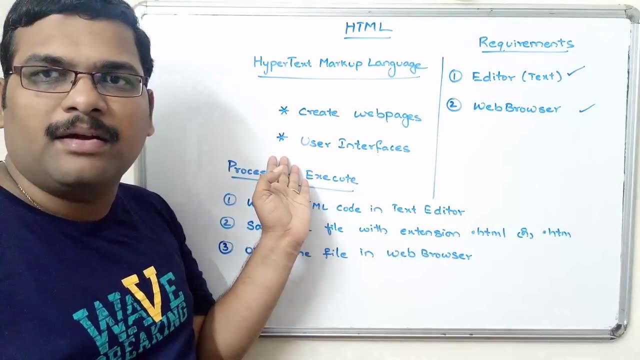 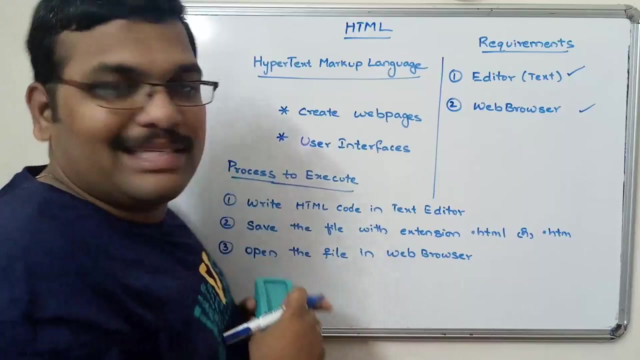 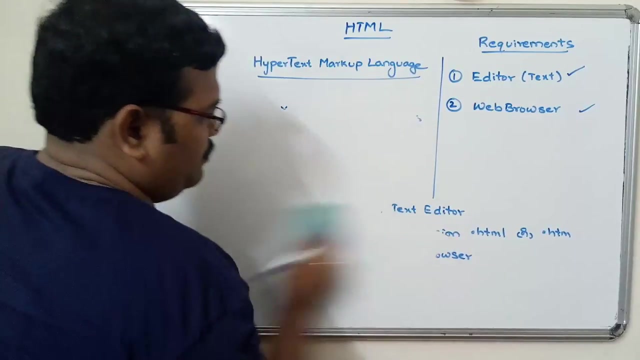 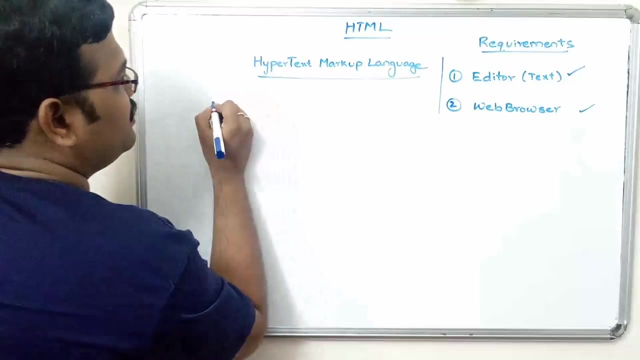 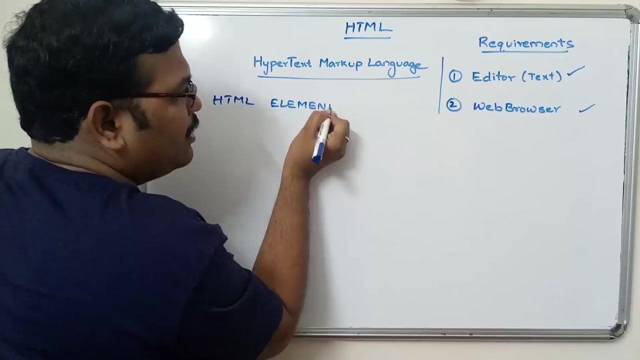 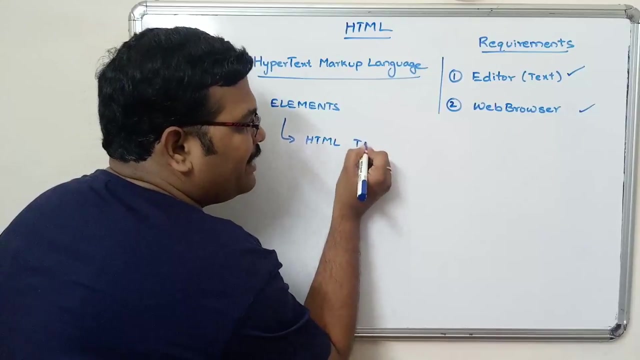 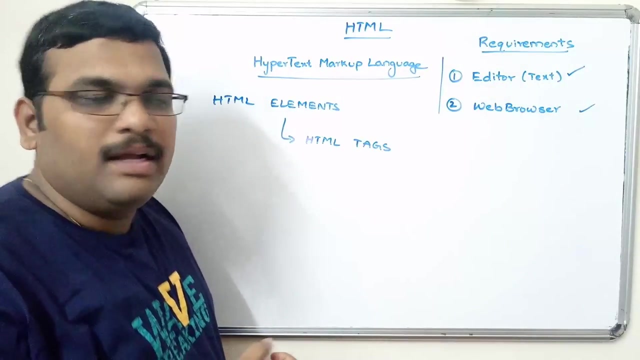 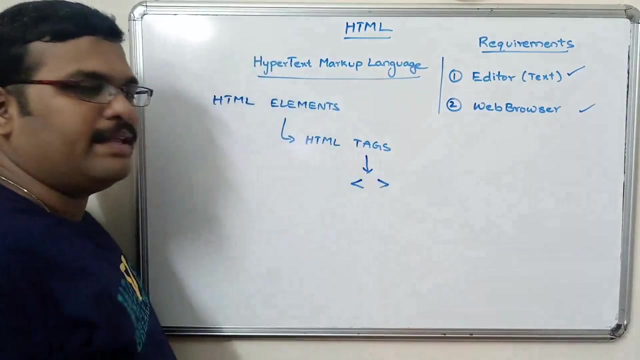 so this is the process and these are the requirements and this is the applications where we will use this hypertext markup language. now, what will be there in this html? so, in this html, the code is written as html elements. elements, right, so html elements. we call them as html tags. so by using these tags, we will write the code. right, so a tag is represented in between the less than symbol and the greater than symbol. 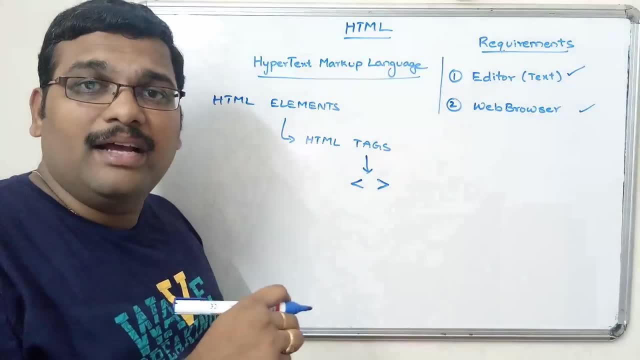 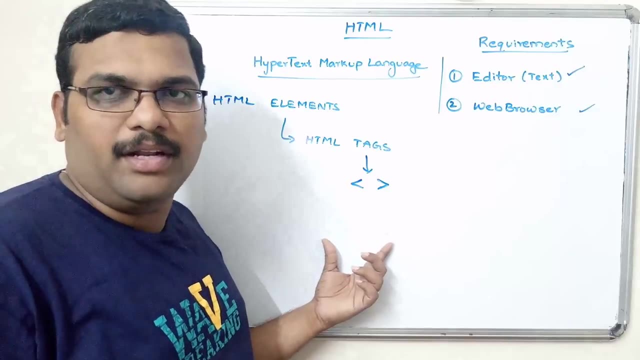 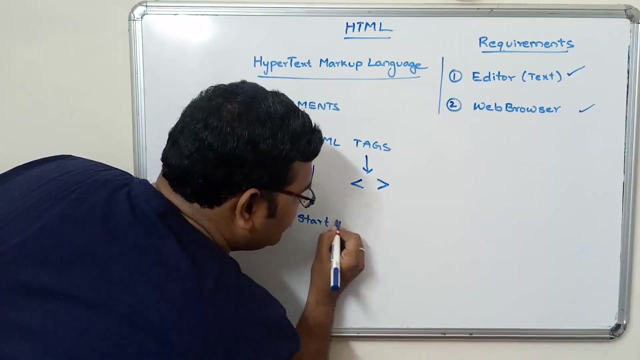 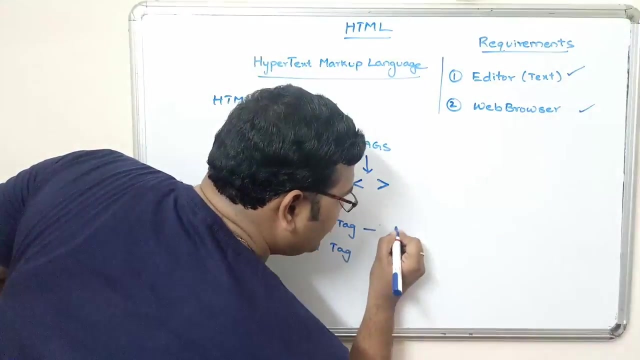 this is very important, so every html tag is represented in between the less than symbol and the greater than symbol. these two delimitus, and every tag will be having Start tag and end tag. start tag is represented as less than greater than.